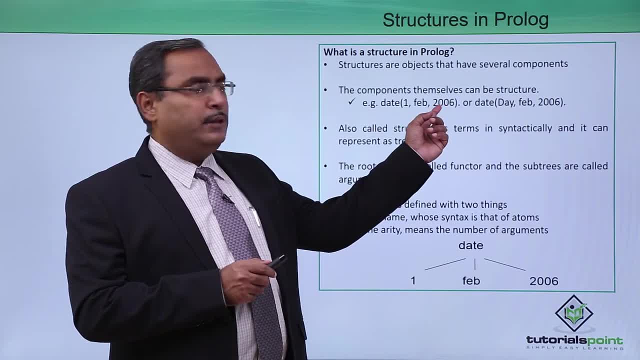 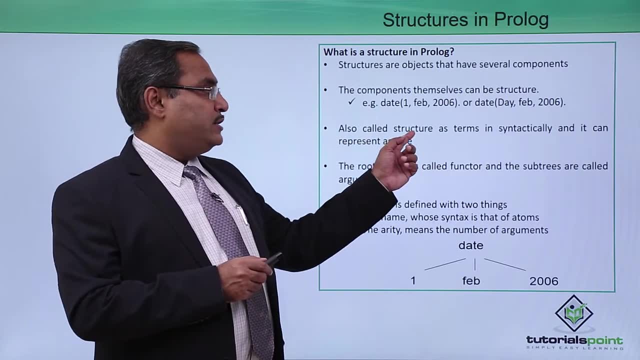 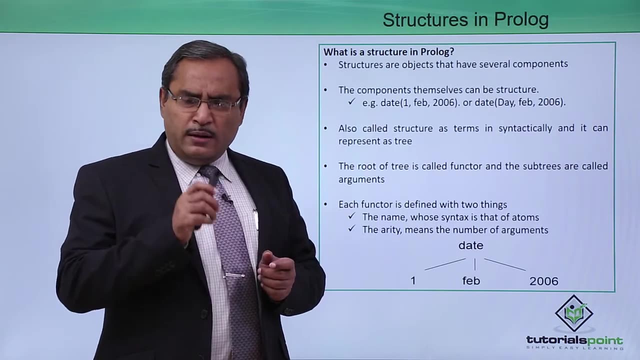 det. Det is a structure because it is having multiple components: are there or det- we can also write in this way, So also called a structure as terms in syntactically and it can represent a tree, While implementing tree in prologue. always we use structures because tree will have. 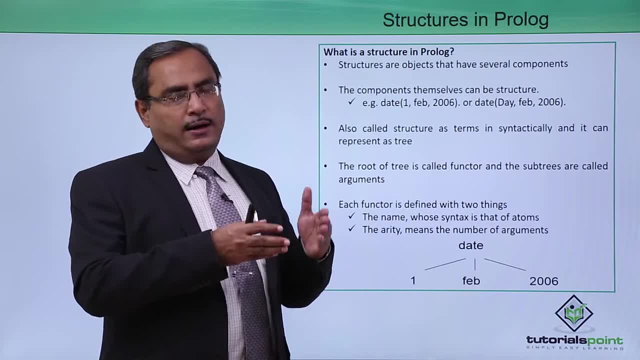 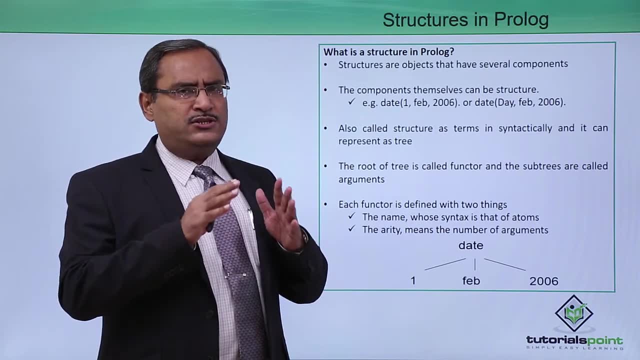 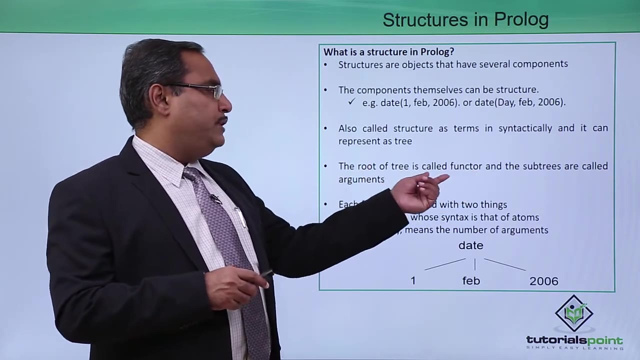 some root node. In case of binary tree, it will have a left subtree, it will have a right subtree. So to represent a tree in prologue, always we use structures. The root of tree is called the functor- Very important term, Remember this one. The root of the tree is known. 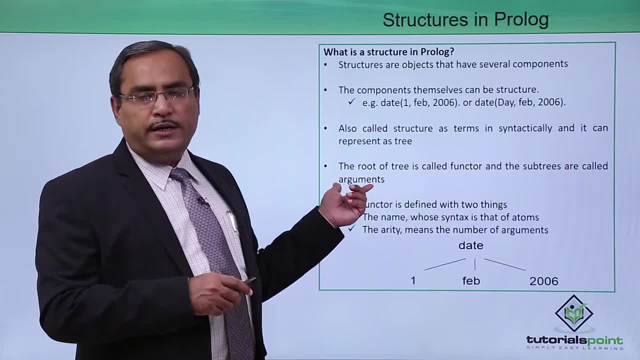 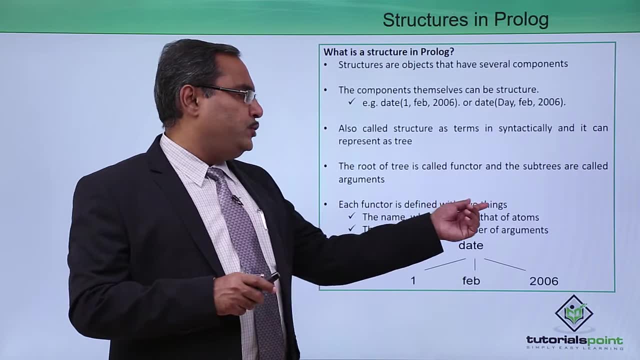 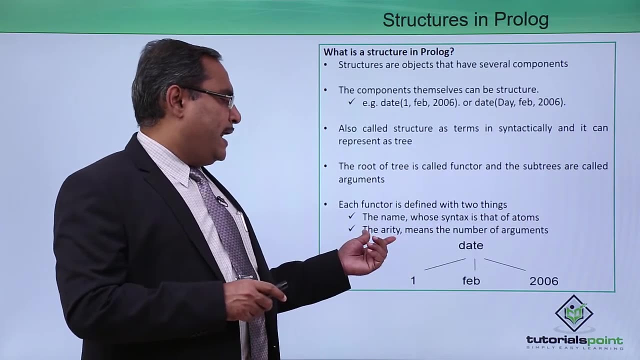 as a functor, and the subtrees are called the respective arguments. So functors and arguments. Each functor is defined within two things: The name, whose syntax is that of the atoms. The arity means the number of arguments. If the things are not clear to you, let me discuss a little bit Det. 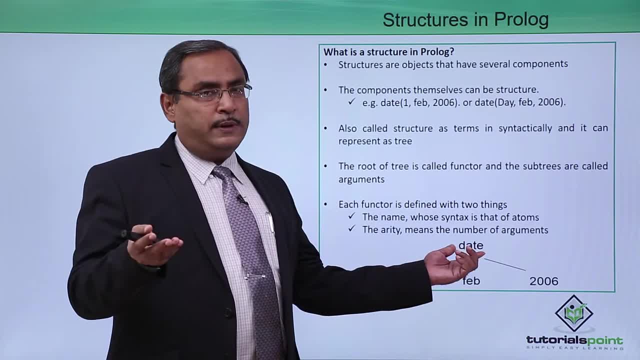 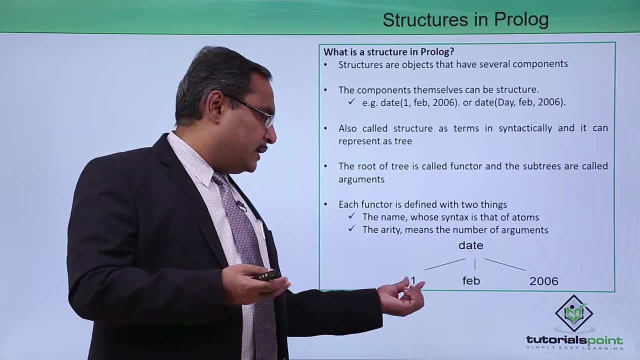 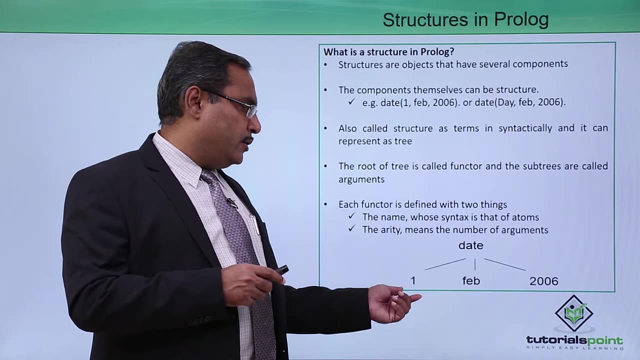 is a functor. So what is a functor? So, whatever the rules are applicable to define an atom, that is same for the functor. So under this functor, these are the respective arguments. How many arguments we are having here? We are having three arguments. So here this arity. 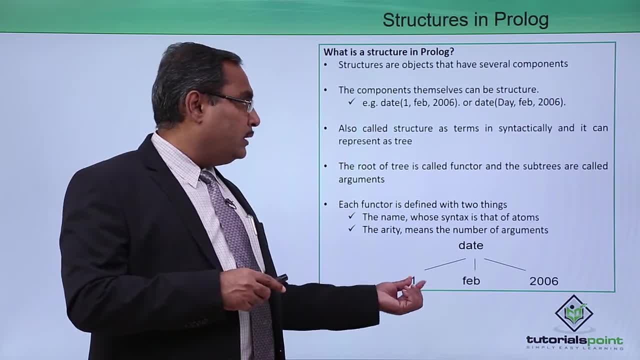 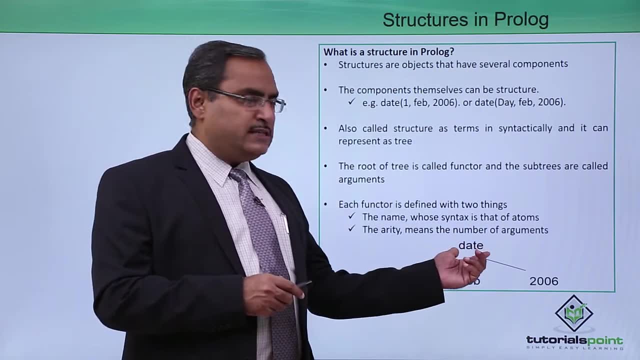 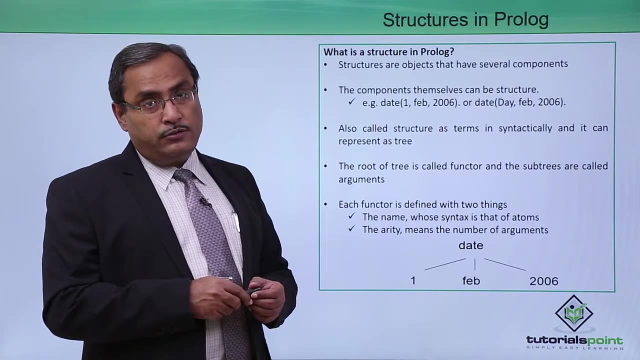 of this functor will be three. So first argument is one, This one corresponding Second argument is fav And the third argument is 2006.. So det is a functor. These are the arguments, And the arity is three here, Because we are having three number of arguments, So let us consider one. 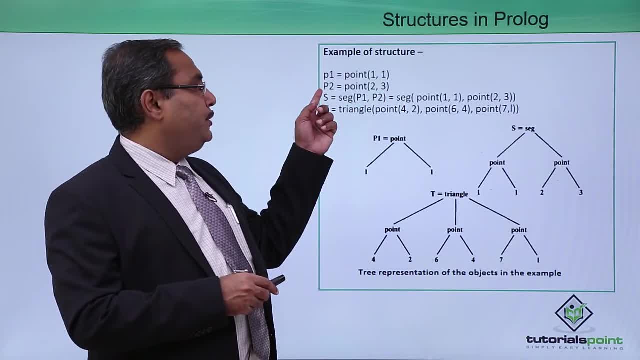 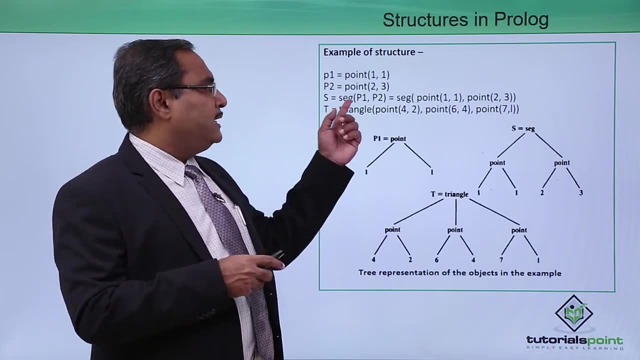 point p1 is equal to point 1 comma 1.. p2 is equal to point 2 comma 3.. So now let us discuss. let us define one line segment. So line segment should have two end points. So p1, p2 can also be written. 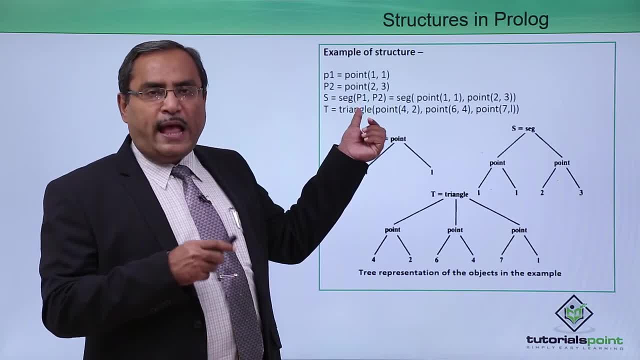 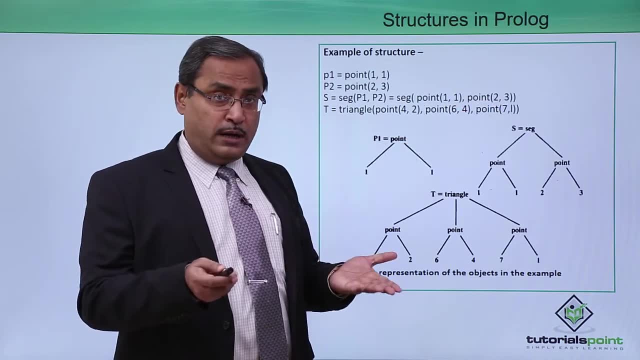 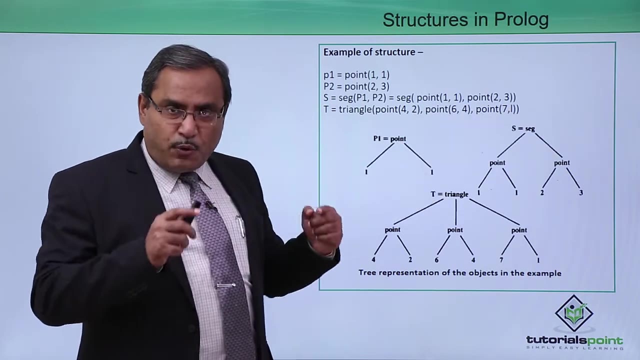 in this way: Here p1 and p2, p are written in capital letters, So they are the variables, But these are functor names and the respective arguments to define p1 and p2.. t is equal to triangle, which is consisting of three points. So three end points are there in a triangle.